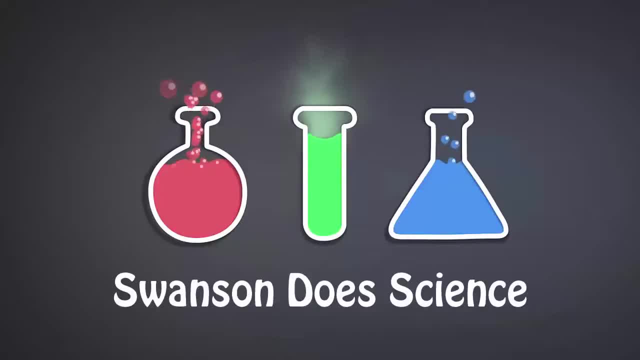 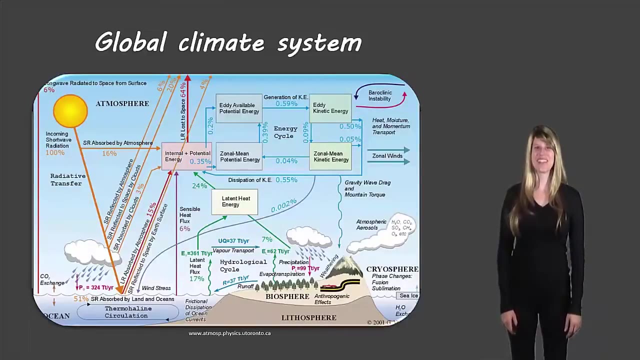 Hello students, Ms Swanson, here and today we have our first lesson in the climate change unit and it's on the global climate system. Now, as you can see from this picture here, the global climate system is a pretty complex thing. We've got convection currents, thermal, 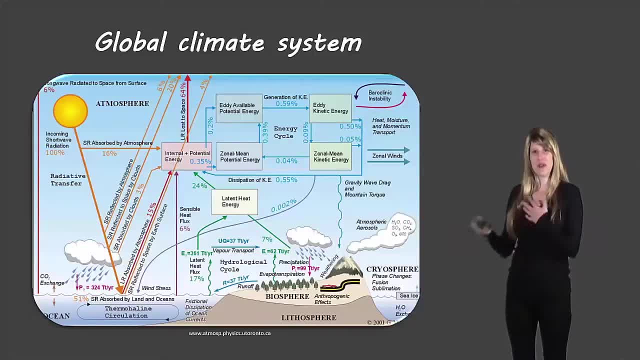 halide circulation, albedo, the absorption and reflection of sunlight. We've got all sorts of things happening there. Now we're not going to learn absolutely everything in this diagram, although we will learn some of the concepts, including those words that I just mentioned now. You'll know what those are by the end of the unit. But what about? 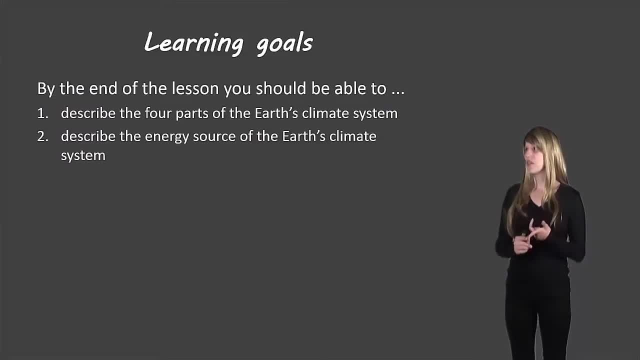 today. These are our learning goals for this lesson: You should be able to describe the four parts of the Earth's climate system and you should be able to describe the energy source for the Earth's climate system. Before we can get into that, let's just talk about the difference between weather and climate. 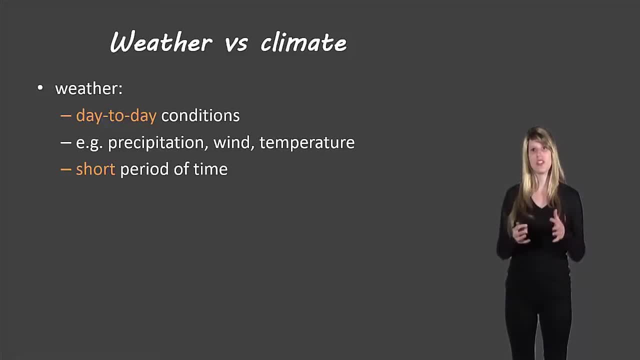 because it is an important difference and sometimes people confuse these two very different concepts. Weather is the conditions over a very short period of time and includes things like temperature, precipitation, wind and so on. So when we talk about weather, we would say what's the weather like today or what's the weather going to be like this week- Climate. 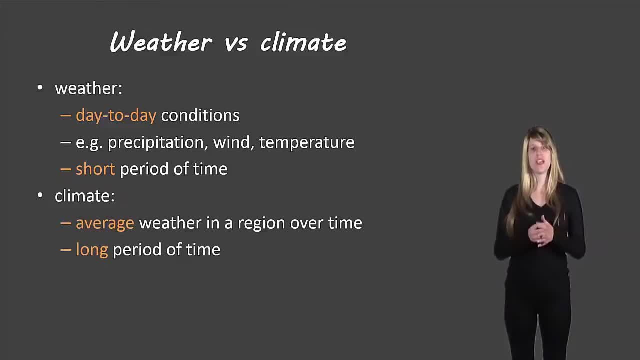 on the other hand, is a very important part of the climate system. The climate system is over a long period of time, For example, over several years or several decades. When we talk about the climate of a certain region, we're still looking at precipitation temperature. 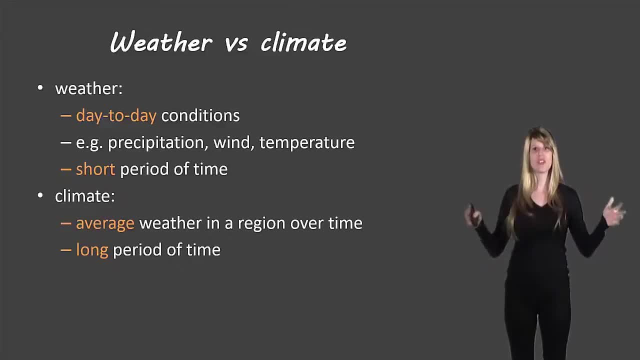 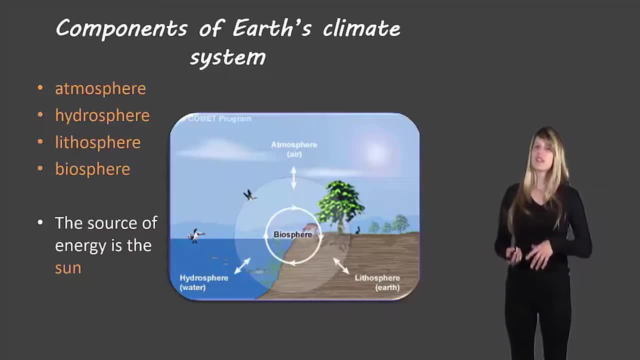 wind and all of those factors, but average temperature or average precipitation over a very long period of time gives us the climate. Now let's get into the components of the Earth's climate system. There are four of them. The first one is atmosphere, and that's the air. 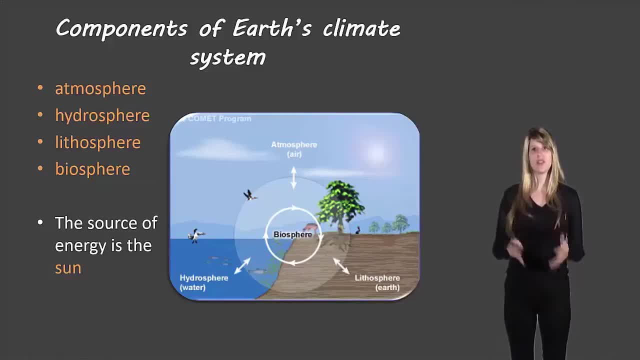 The next is hydrosphere, And that's the water. That includes liquid water, water that's in the gas form or the solid form. Lithosphere, which is the ground, and that includes not just what we're standing on now but the ground underneath the oceans and that sort of area, And then the biosphere.